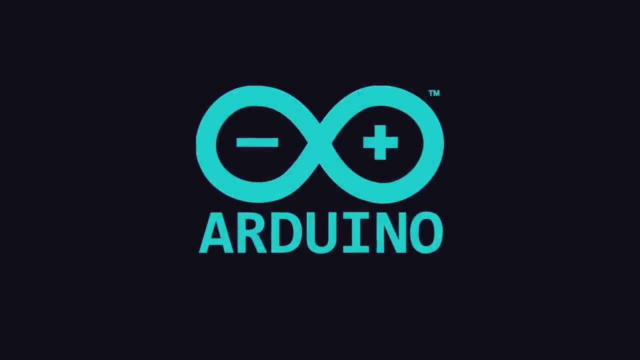 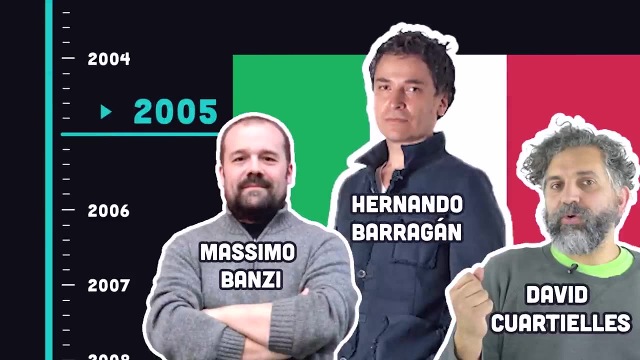 Arduino, an open source programmable circuit board and microcontroller that makes it possible for anyone to build digital hardware products. The idea started in Italy in 2005 and today has sold over 10 million boards worldwide. The most popular model is the Uno, and at its heart we have a: 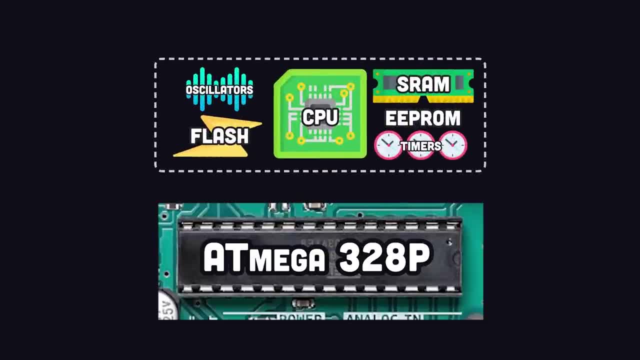 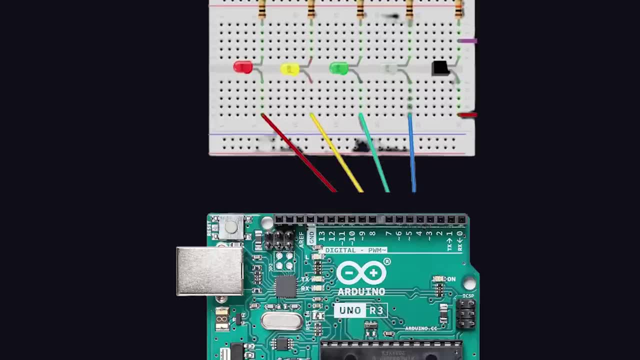 microcontroller, which is like a small, inexpensive computer that can run on low power. The board is surrounded by pins that can be used to construct a circuit by connecting various input and output devices. Most importantly, though, it has a USB port that's used to easily upload your code to. 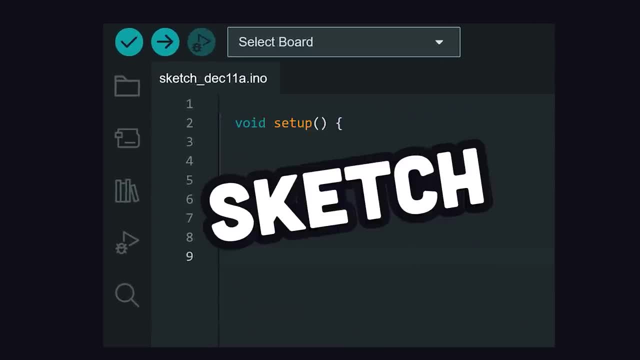 the device. In Arduino, a software program is called a sketch, which is written in a purpose-built, easy-to-learn programming language. Every program has two basic functions: Setup runs once when the hardware is first powered on, and loop runs continuously to react to signals from input. 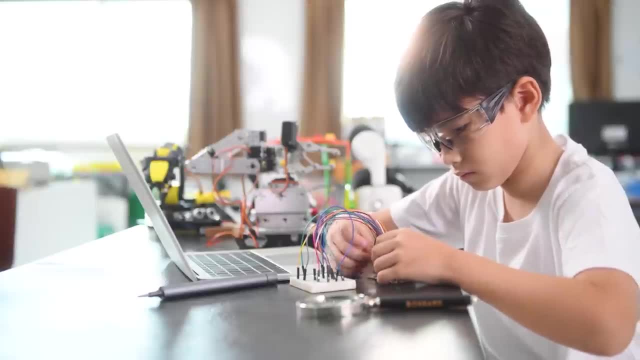 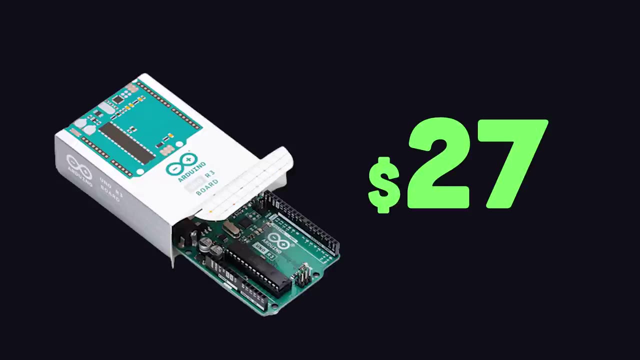 devices or changes to the state of the program. Arduinos have been used to build IoT products, robots, wearable devices and all kinds of other crazy hardware ideas. To get started, I'm going to show you how Arduino works. To get started, obtain a board, then download its custom IDE or use the VS Code plugin if you. 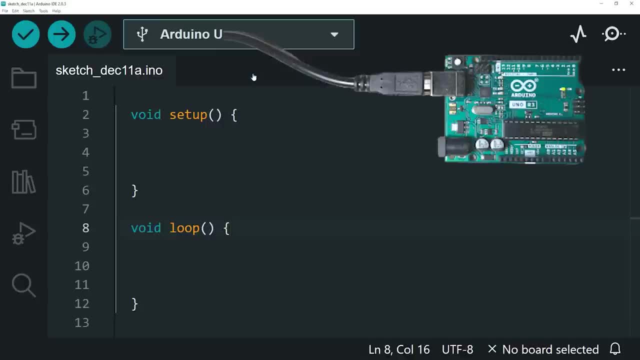 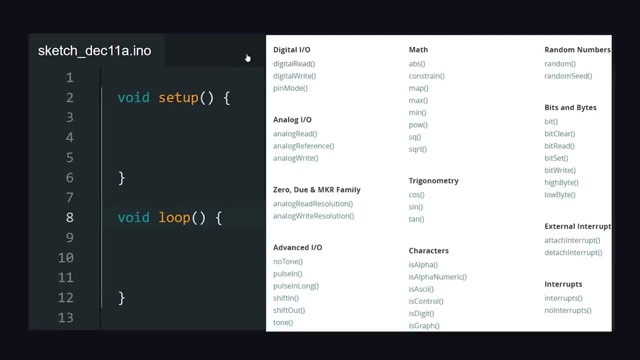 prefer, Once installed, connect your board via USB, then create a new sketch, which is just a file ending in ino. The language itself feels like a simplified version of C with plenty of built-in functions to make hardware coding more accessible. The setup function runs once, when the 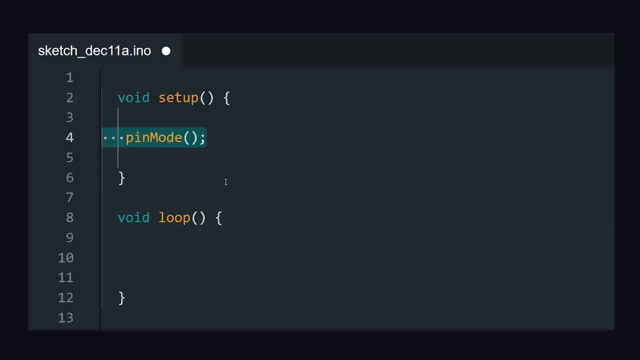 board is reset or powered up, We could use the built-in pin mode function to select a pin like the built-in LED and then configure it as an input or output. And now in the loop function we can turn the LED on and off. 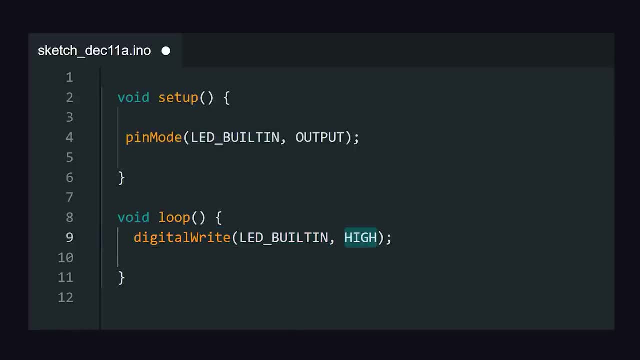 We can turn the LED on by writing to it with a value of high, which is a constant. that will increase the voltage to that pin and make it shine, To make it blink. we can follow it with a delay, then switch the voltage to low And now we can hit the upload button to compile and run. 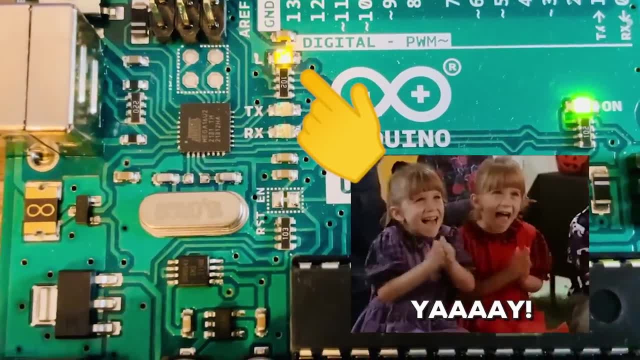 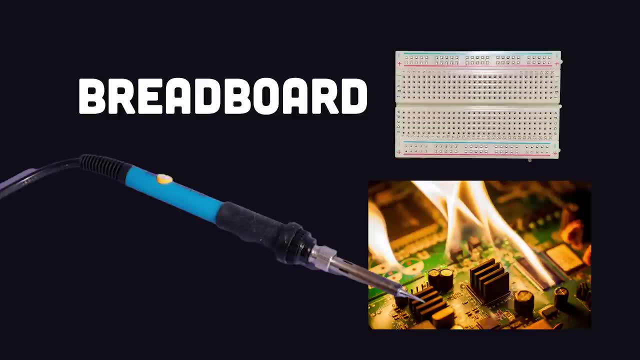 this code on the Arduino's microcontroller. Congratulations: you just built a custom hardware product, But there's a lot more we could do here. Connect a breadboard to it to create circuits without the need for soldering. The Arduino can power it by connecting the positive.